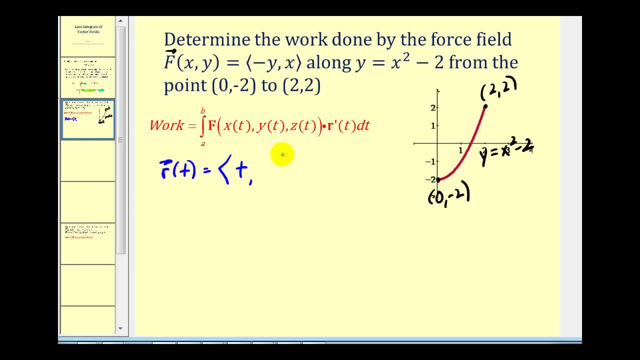 squared minus two. we could let the y component equal t squared minus two And the interval for t would be from zero to two. Let's go ahead and set up our def integral in terms of t. The momentum integration will be from zero to two. We'll rewrite our 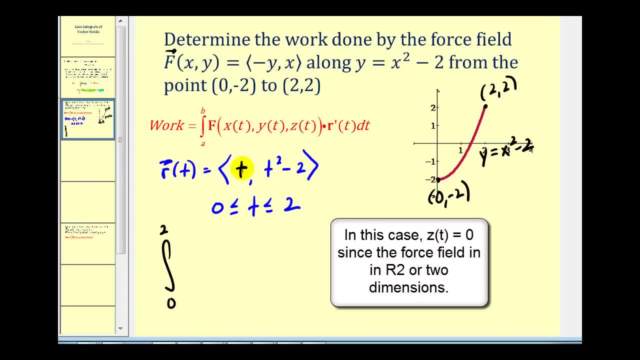 vector field as a function of t, using x of t and y of t. So the x component will be the opposite of y of t. Well, here's y of t. so instead of t squared minus two, it'll be two minus t squared. 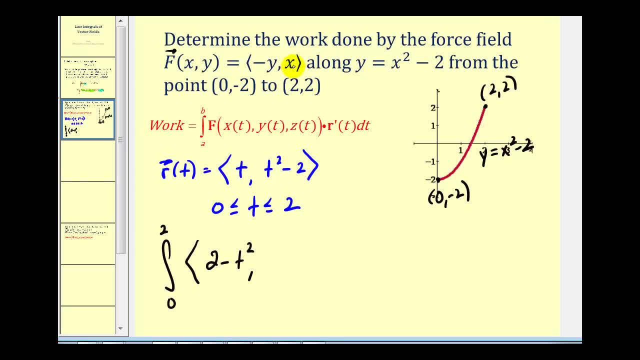 For the y component is equal to x, x of t is equal to t, And we'll dot this with r, prime of t. So we'll have one and two t- Let's go ahead and evaluate this on the next page. So we'll have two. 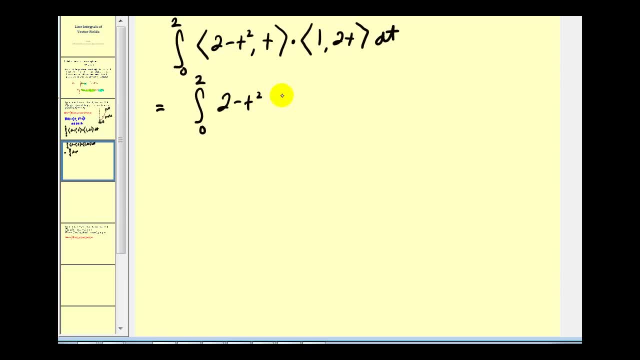 minus t squared times one, That's two minus t squared. Plus t times two t, That'll be two t squared. Let's go and combine our like terms. We'll have two plus t squared, So we'll have two t plus one, third t cubed. So when t is two, we'll have four plus two plus one. 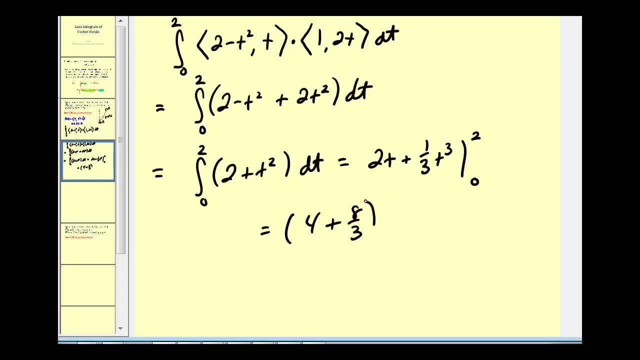 four plus this will be eight-thirds. And then, when t is zero, these are both zero. Well, four is equal to 12-thirds, so that'll be 20-thirds, So the work is 20-thirds. Let's take a look at the given path in this force field. 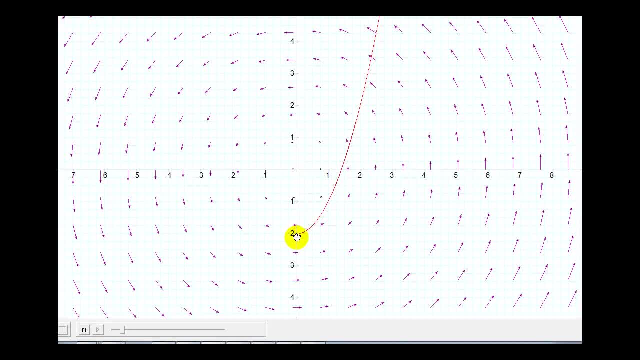 So here we see the force field, and the path we're taking is from this point here to the point two. two Now notice how the vector field is moving counterclockwise and the path is also moving counterclockwise, And that's the reason why the work is positive. 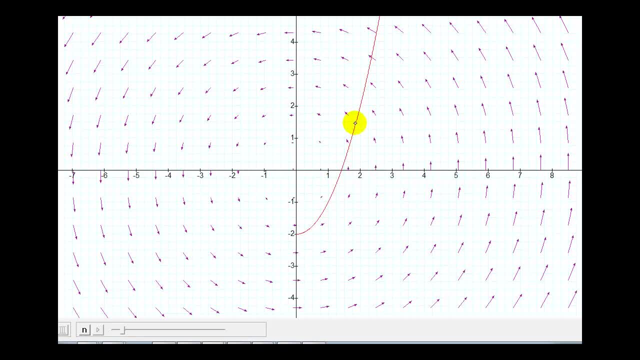 If the motion is in the same direction as the force field, the work will be positive, And if it's in the opposite direction of the force field, the work should be negative. Now notice for this example: our force field was two-dimensional. 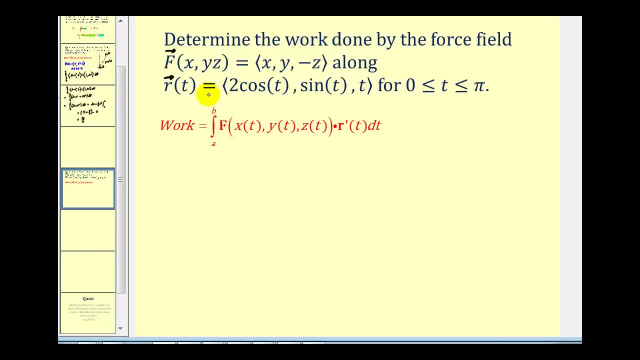 and now we'll take a look at one that's three-dimensional. So it's the same question, but now we have we have a three-dimensional force field and our path is now a space curve rather than a plane curve, But the process will be exactly the same. 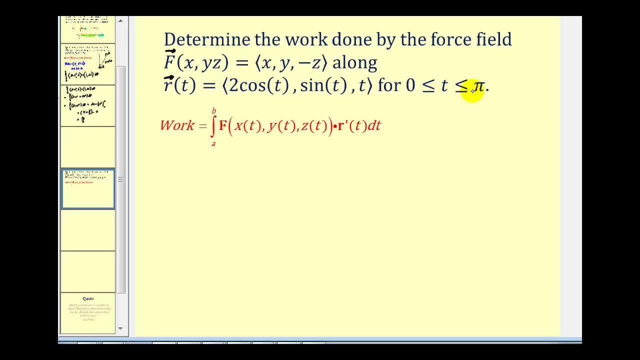 And for this example, we already have r of t as well as the interval for t, so we can go ahead and set up our definite integral in terms of t. Limits of integration will be from zero to pi When we write the given force field as a function of t. 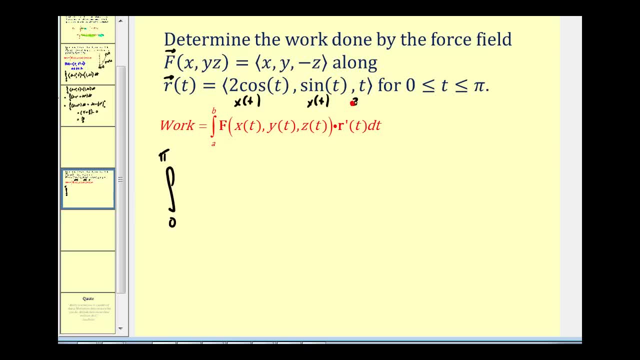 using x of t, y of t and z of t. So the x component is equal to x. that'll be two cosine t. The y component will be y, so it's still sine t And the z component is the opposite of z. 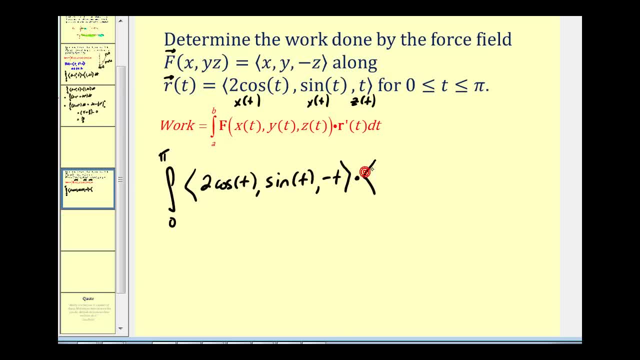 so that'll be negative t, And we'll dot this with our prime of t, So we'll have negative two sine t, cosine t and one. So we'll have negative four: cosine t sine t plus cosine t sine t. 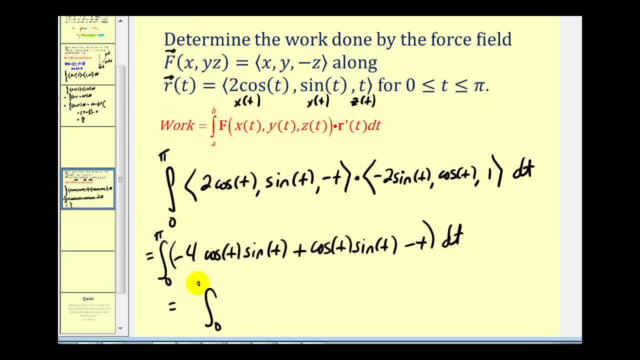 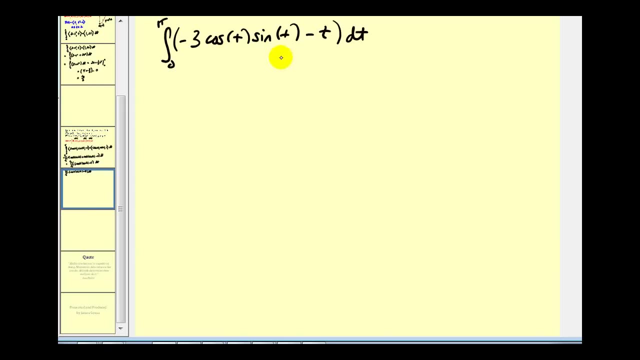 minus t. Let's go ahead and combine our like terms. We have negative three: cosine t, sine t, minus t and sine t, And let's go ahead and finish this on the next page. And to integrate this, let's go ahead and let u equal cosine t. 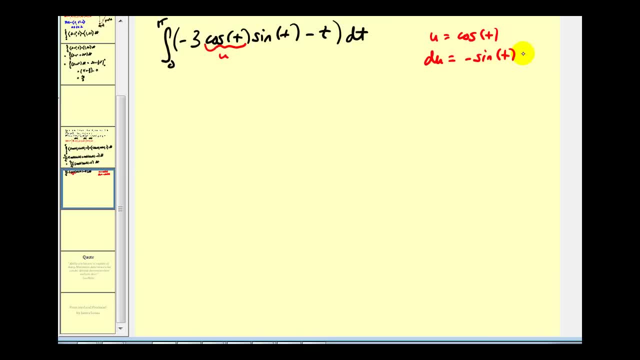 So differential u is going to be negative sine t dt. Notice we do have a factor of negative sine t dt. So this just simplifies to three u. So we'll have three times u squared over two or three halves cosine t squared. 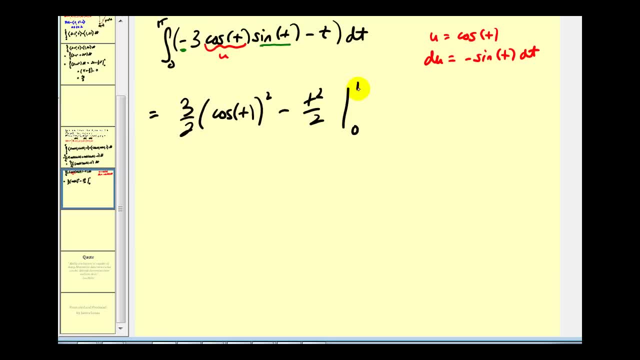 then we'll have minus t squared over two. First evaluate this at pi. Well, cosine pi is equal to negative one. Negative one squared is one. So we'll have three halves, then minus pi squared over two. And then, when t is zero,